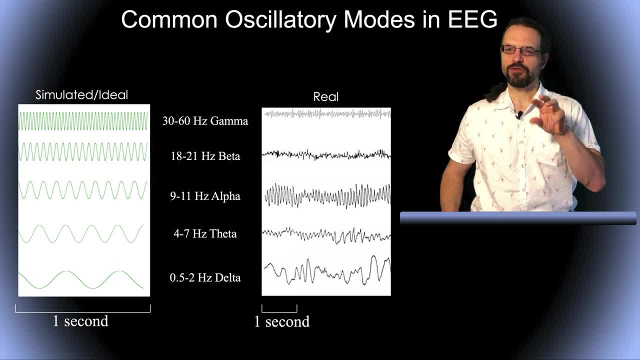 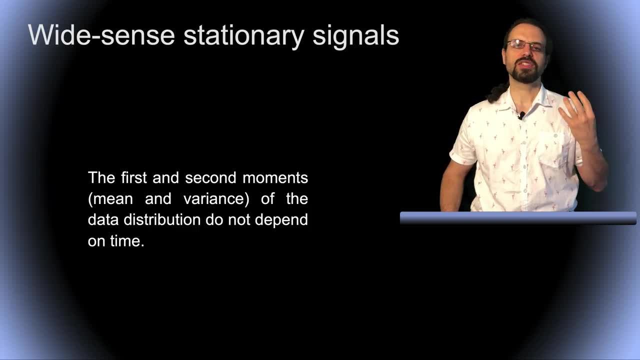 So now we are going to see how we can extract the frequency content of the EEG signal, And for this we need to make the assumption that the EEG signal is stationary. So this is not entirely true for the EEG signal, but it's approximately true over short time windows. 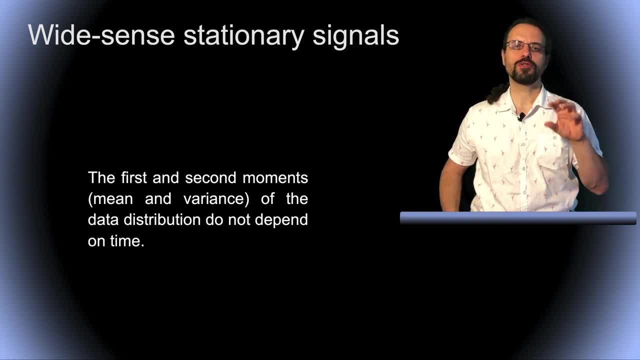 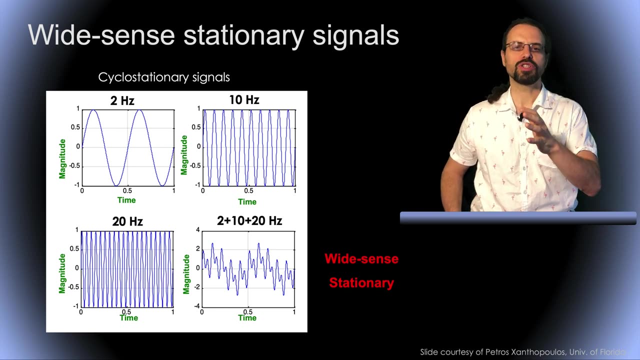 And by stationary we mean that the first and second moments, so the mean and the variance of the data distribution doesn't depend on time. So let's look at an example Here we have different stationary sinusoids, one at 2 Hz, one at 10 Hz, one at 20 Hz. 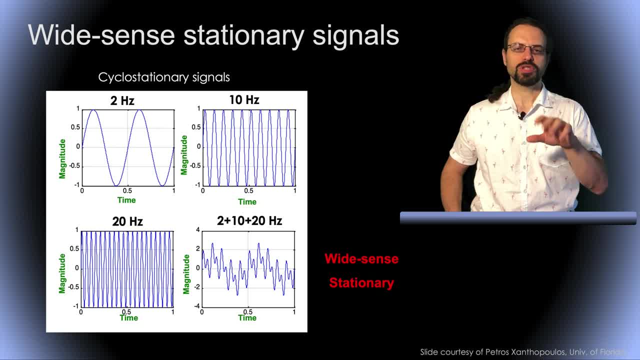 If we simply add this signal, as this is represented in the bottom right corner, you can see that this signal has a complex feature And it is stationary because it is a sum of stationary signals. Now, if we want to analyze this signal, to see what the signal is made out of, 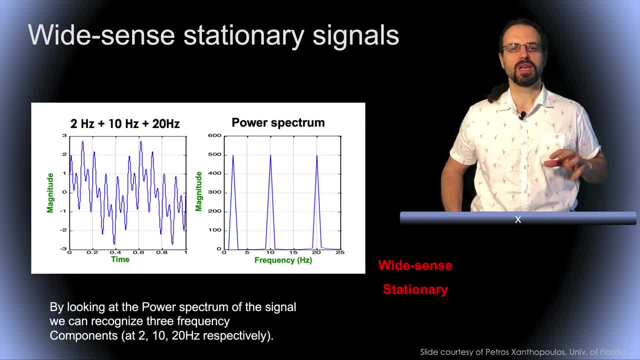 we can perform a power spectrum. By looking at the power spectrum of the signal, we can recognize three frequency components of the signal at 2, 10 and 20 Hz. So in the next slides we're going to see how to build such a power spectrum. 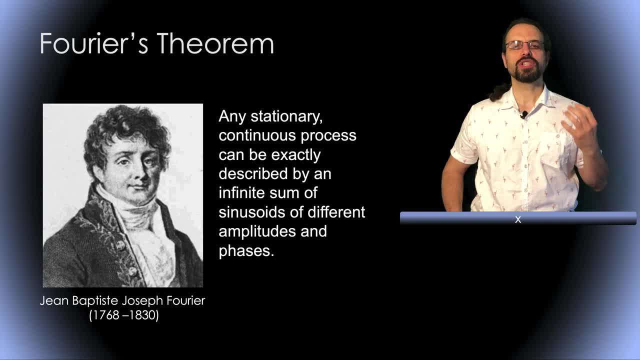 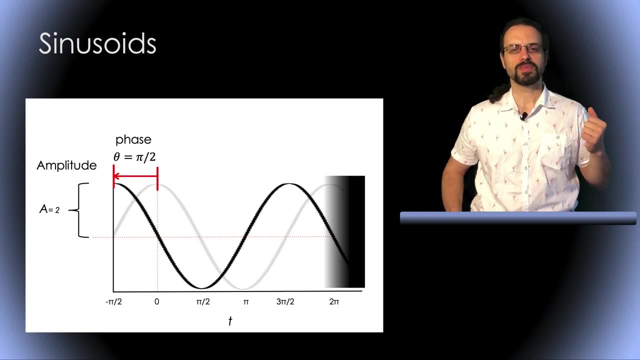 So Fourier stated that any stationary continuous process can be exactly described by an infinite sum of sinusoids at different amplitudes and phases. So let's first define what we mean by amplitude and phase of a sinusoid. Here is a sinusoid and the amplitude is the height on the y-axis. 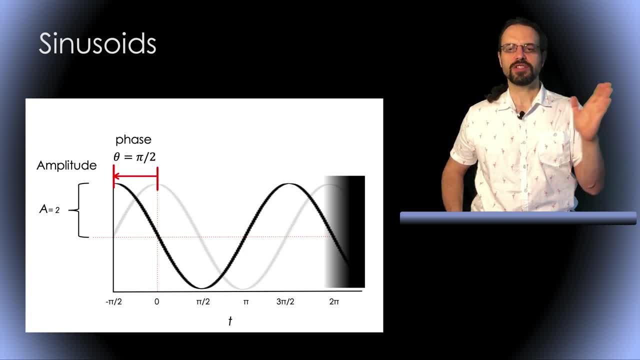 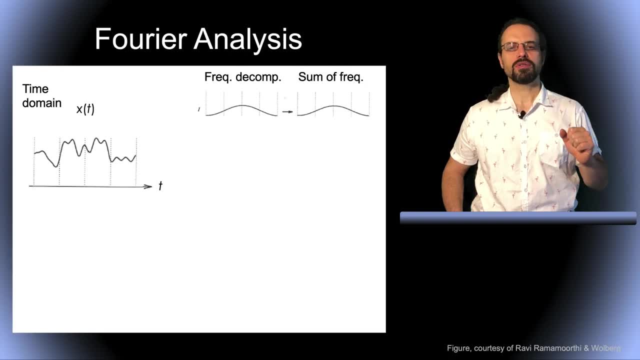 and the phase is the shift of the sinusoid on the x-axis. So here we have a signal in the time domain on your left and a frequency decomposition of this signal on your right. We only have one frequency here, but we're going to add some more. 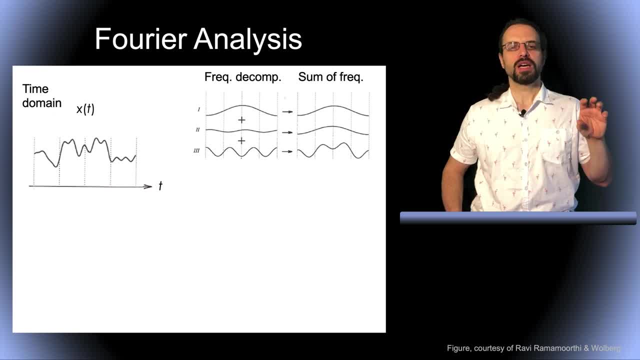 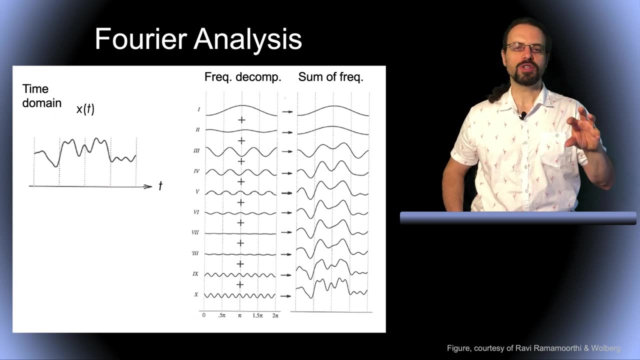 So now we have three different frequencies with different phases and amplitudes, And you can see that as we sum over these frequencies, the original time domain signals start to appear. When we use more frequencies of different phases and amplitudes, we can recover at the bottom right the original signal. 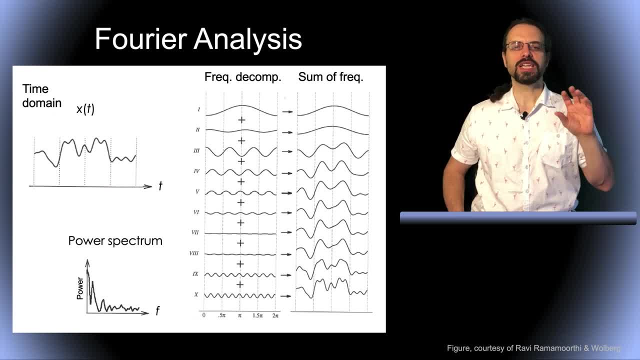 We can then construct the power spectrum by just looking at the amplitude at different frequencies. So at this frequency the amplitude is relatively high, so we have a peak in the power spectrum. At this other frequency, the amplitude is very low, so we have a trough in the power spectrum. 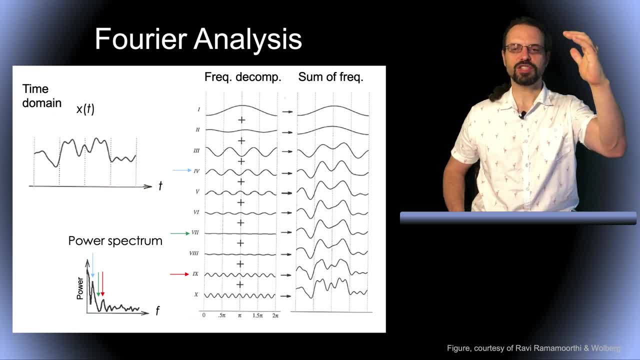 And at this third frequency the amplitude is high again. so we have another peak in the power spectrum. As a side note, the power spectrum is actually not the raw amplitude, but the square of the amplitude of all these frequencies. So this is how the power spectrum is built. 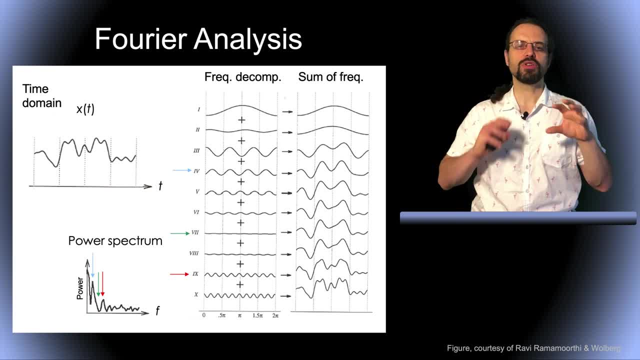 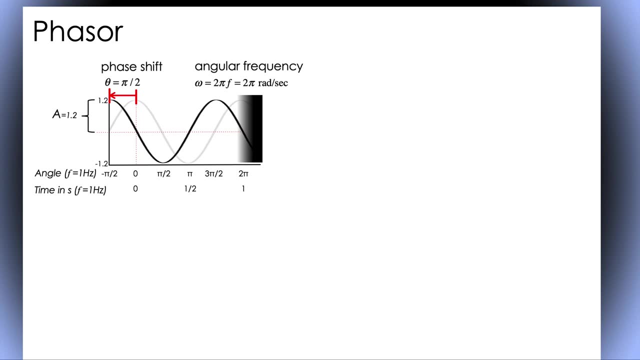 And the goal of Fourier analysis is to learn the correct amplitude and phases for each sinusoid, such that their sum reconstructs the original time series. So, a little bit formally, we already saw the amplitude and phase shift of a sinusoid And this is the equation describing the sinusoid. 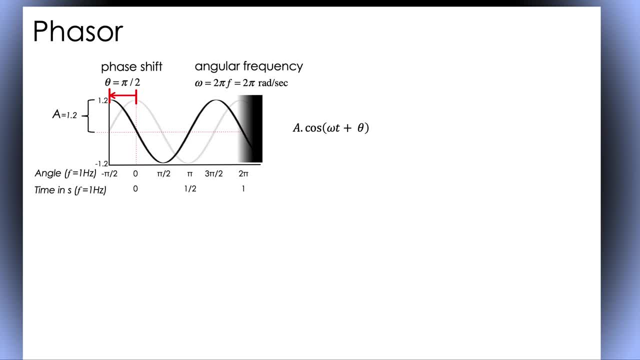 When dealing with a sinusoid, we usually use the angular frequency, which is equal to 2 pi times the frequency in Hertz, And this cosine formula is equal to the real part of this complex exponential. This is Euler's formula, And this complex number is called a phasor. 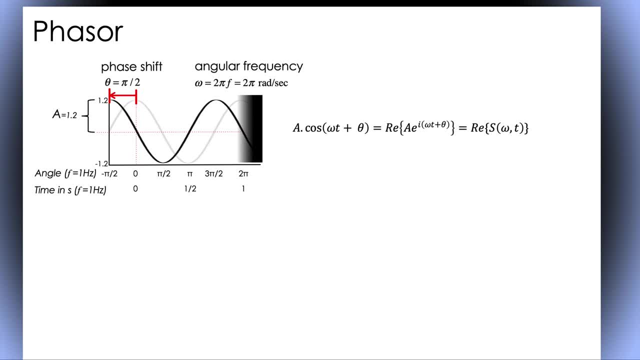 sometimes represented by s of omega and time. So a phasor may be represented with a vector and the length of the vector represents the amplitude and the angle of the vector represents the phase. So you might have seen this other notation from Euler's formula. 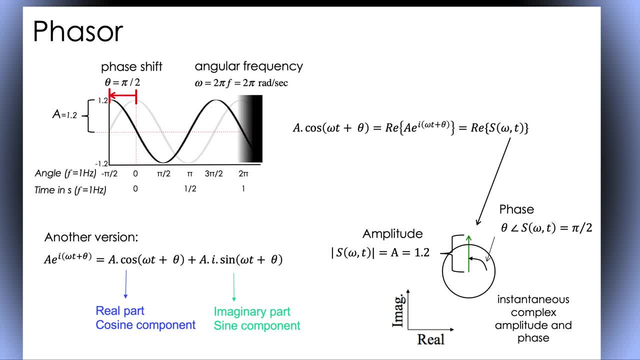 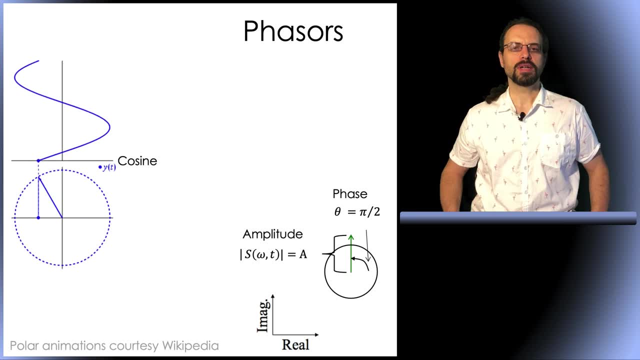 in which a complex exponential can be decomposed into a real cosine part and an imaginary sine part. So let's see an example here. This is the phasor that we just talked about, And as time increases we can see the phasor rotates. 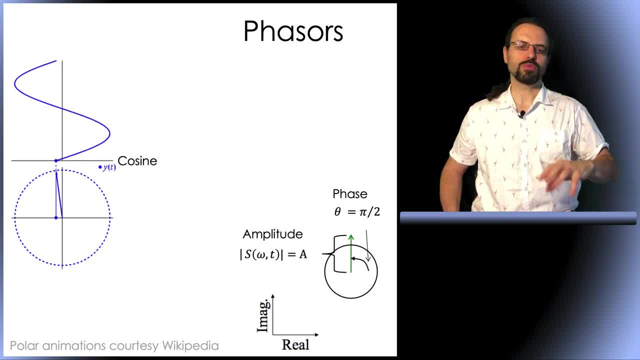 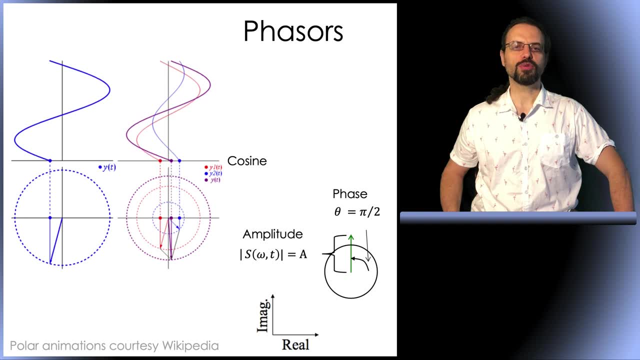 And this is the representation of the real part of the phasor, which is the cosine. And here is another representation with three phasors, and the purple being the sum of the red and blue phasors, And we can see different phase and amplitude of this phasor.